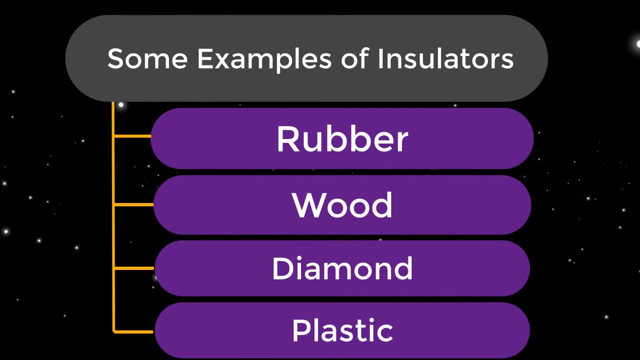 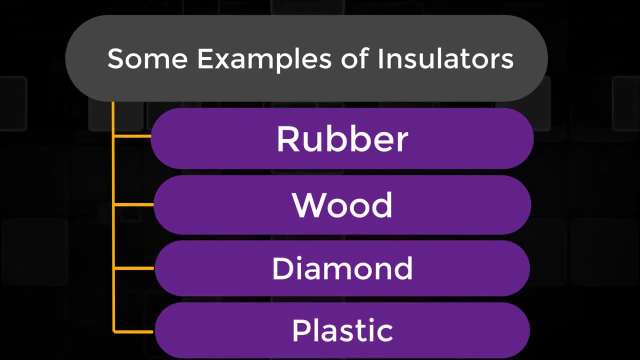 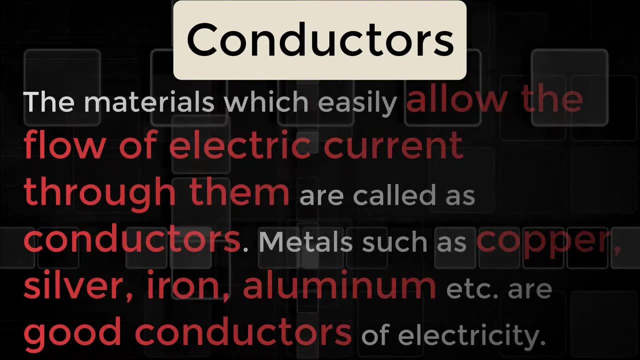 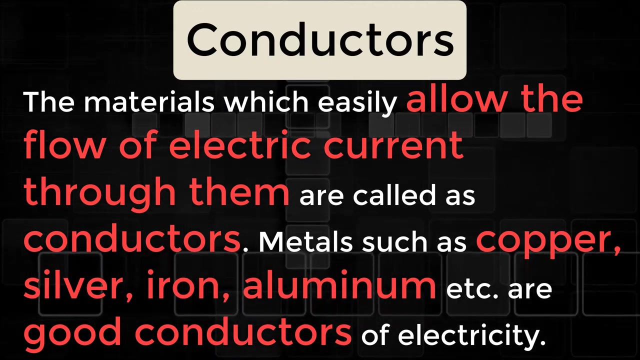 as plastics, are used for coating of electrical wires. These insulators prevent the flow of electricity to unwanted points and protect us from electric shocks. Conductors- The materials which easily allows the flow of electric current through them, are called conductors. Metals such as copper, silver, iron, aluminium, etc. are good conductors. 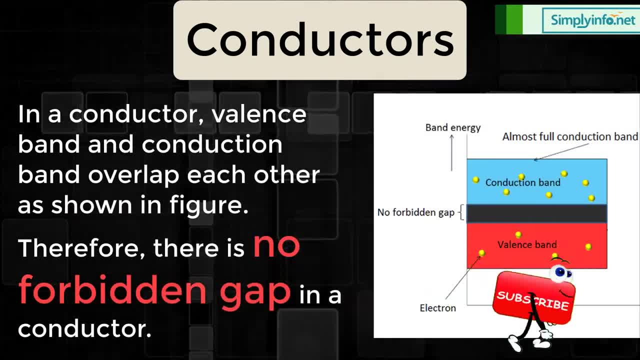 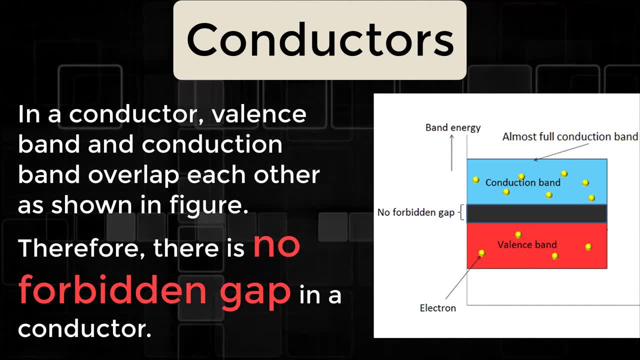 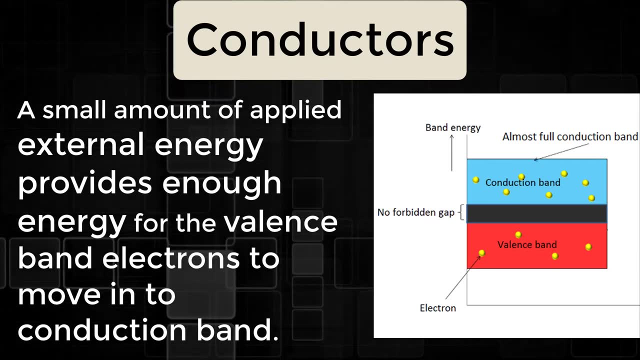 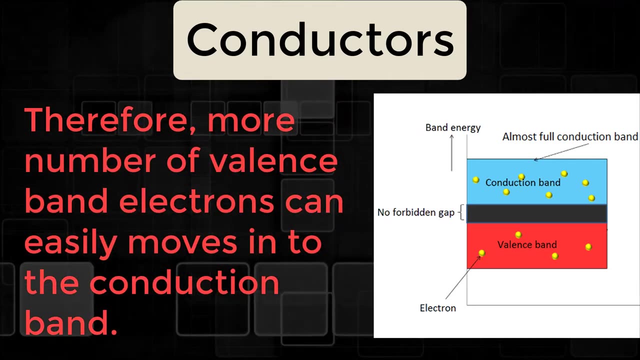 of electricity In a conductor, valence band and conduction band overlap each other. Therefore there is no for balanced gap. A small amount of applied external energy provides enough energy for the valence band electrons to move in conduction band. Therefore more number of valence band electrons. 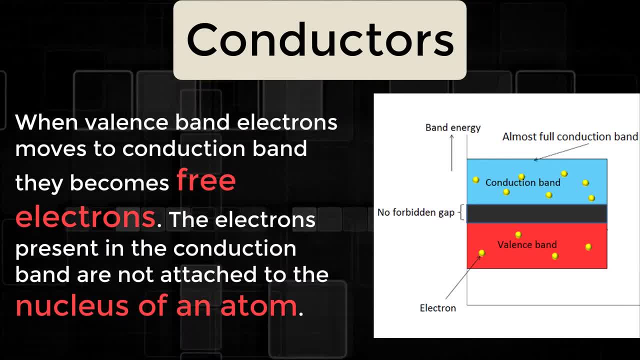 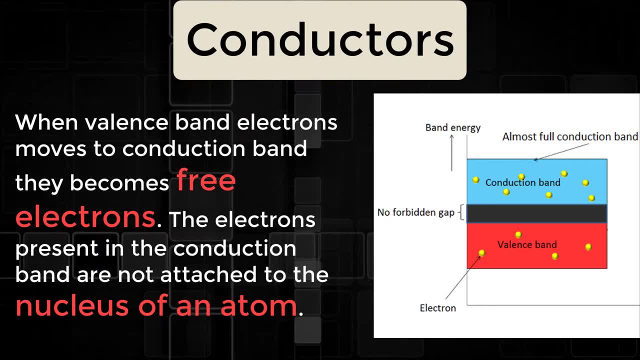 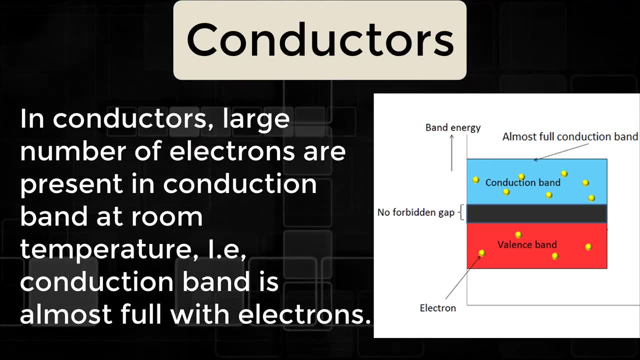 can easily move into conduction band. Valence band electrons can easy glasses cause? the electrons present in conduction band to band are not attached to the nucleus of an atom In conductors. large number of electrons are present in conduction band at room temperature. 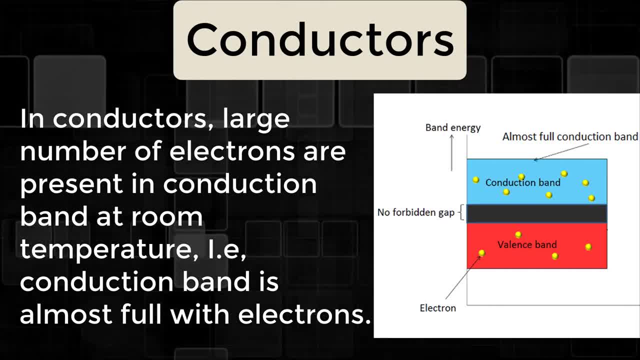 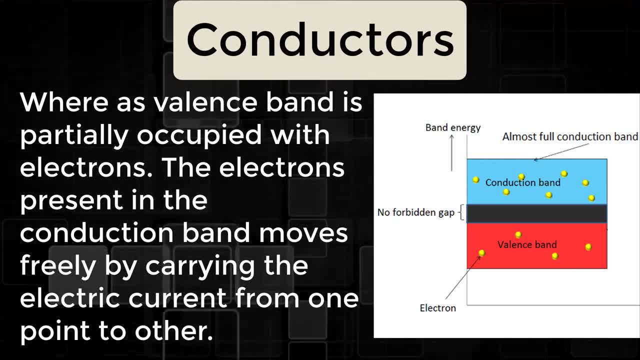 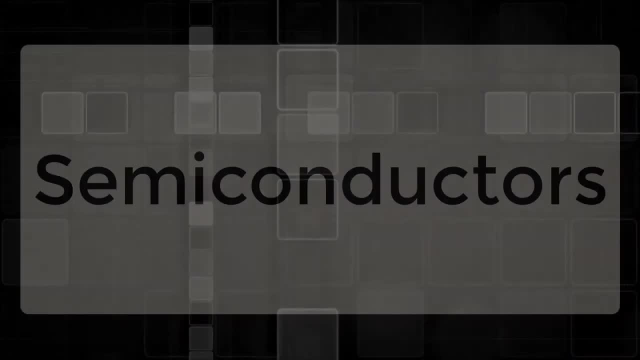 That is, conduction band is almost full with electrons, whereas valence band is practically occupied with electrons. The electrons present in the conduction band moves freely by carrying the electric current from one point to other. Now let's look into semiconductors. 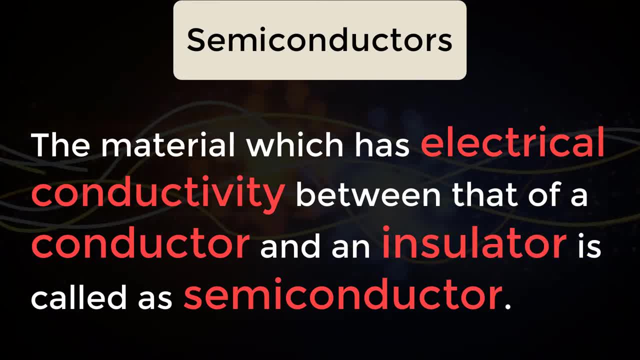 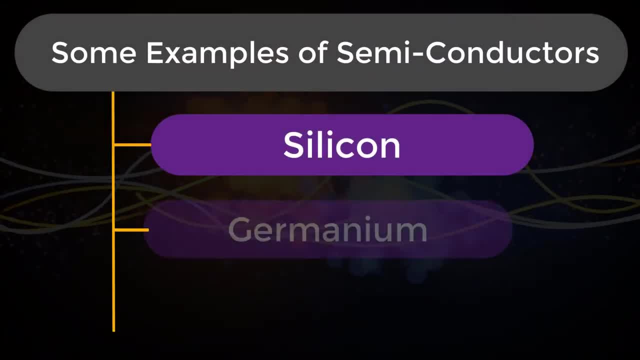 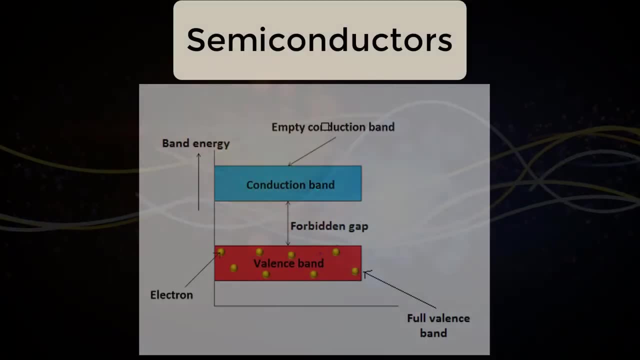 The material which has electricity conductivity between that of a conductor and an insulator is called a semiconductor. Silicon, germanium and graphite are some examples of semiconductors. In semiconductors the fibrin gap between valence band and conduction band is very small. 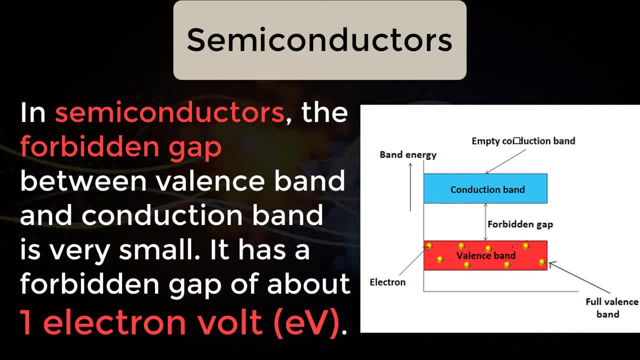 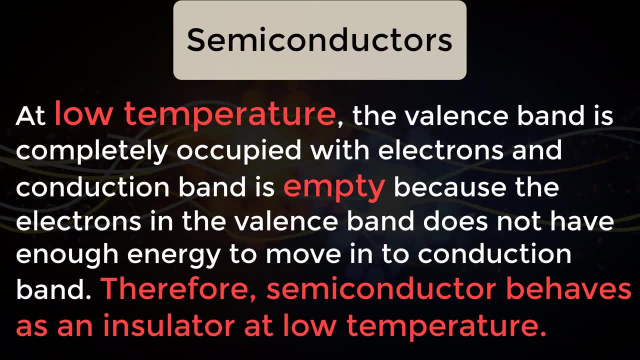 It has a fibrin gap of about 1 electron. The fibrin gap between a conductor and an insulator is about 1 electron. At low temperature the valence band is completely occupied with electrons and conduction band is empty because the electrons in the valence band does not have enough energy to move into.